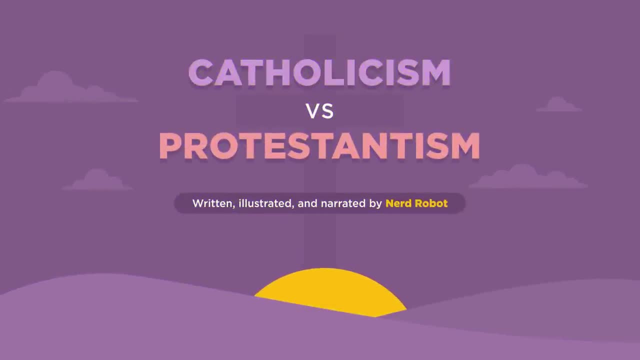 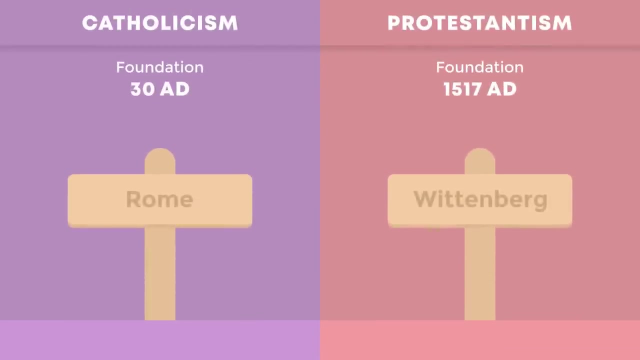 Hey there, today we're going to chat about something pretty interesting: Catholicism and Protestantism. We'll take a look at what sets them apart, what they've got in common and why it even matters. So stick around. Catholicism has its roots in Rome, around 30 AD, shortly after Jesus Christ's crucifixion. 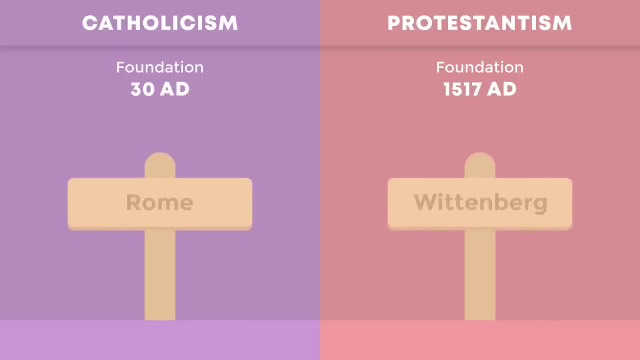 The early Catholic Church viewed itself as the continuation of Jewish law and the teachings of Jesus Christ passed on to the Apostles. Protestantism, on the other hand, didn't come into existence until 1517 AD, when Martin Luther, a German monk, initiated the Protestant. 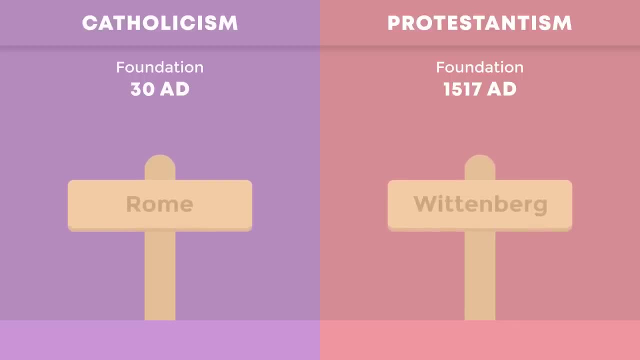 Reformation in Wittenberg, Germany. This was an attempt to reform perceived corruptions within the Catholic Church which, according to Luther and his followers, had deviated from the original teachings of Christianity. St Peter, a prominent Apostle of Jesus Christ. 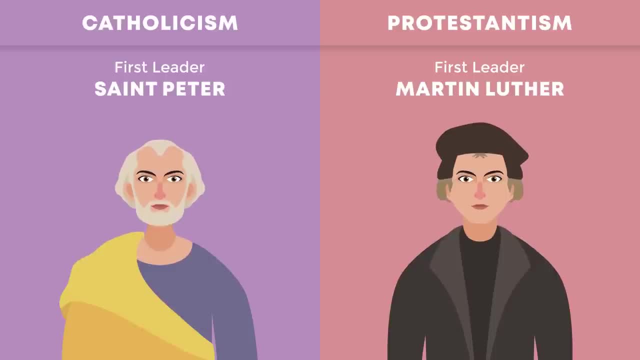 is traditionally considered the first leader or pope of the Catholic Church. According to Catholic belief, Peter received the keys to the Kingdom of Heaven, making him the leader of the earthly Church. In contrast, Martin Luther, a German monk, theologian and professor, sparked the Protestant Reformation in the 16th century. 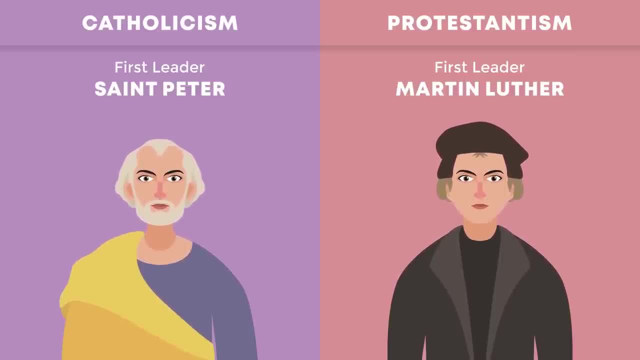 and is therefore often seen as the first leader of Protestantism. He was instrumental in developing a theology that emphasized faith, scripture and religion. He would demonstrate the ultimate most他们's unique God, the One Almighty God, who was known to all as the King of Heaven, who had crowned heaven and earth in the sky and 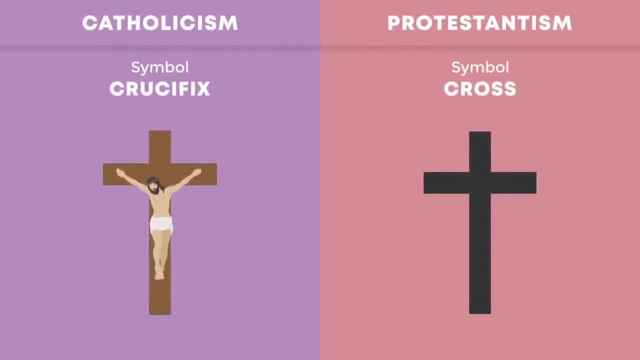 who was known as One of the Giants, one of the mostames of the religious hierarchy. He was also an important leader of Protestantism and the Catholic Church. He was an important leader of Protestantism and the Catholic Church, as well as an important 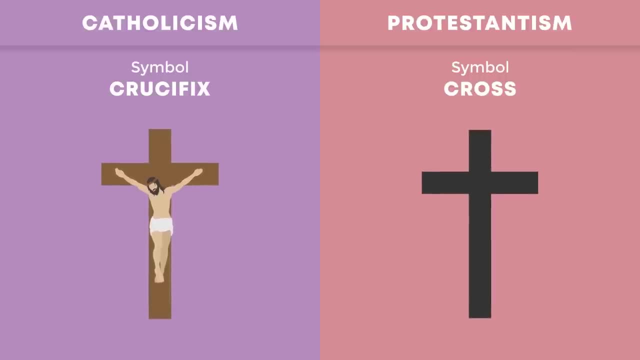 leader of the Christian faith. The Orthodoxy, however, was primarily built upon the social, moral, religious and religious matters of the Catholic Church. It was the faith that is most strongly rooted within the Catholic Church, the faith of the Catholic Church and the belief in the Catholic Church. 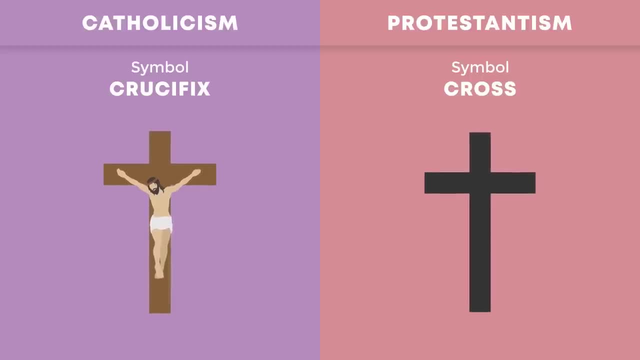 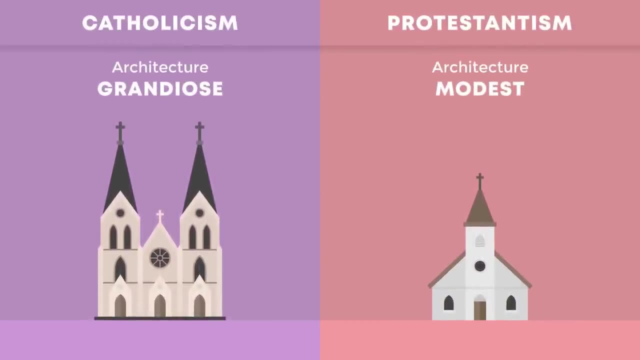 This is the most significant or memories that the Catholic Church has ever made in its history over death and sin, rather than the suffering. the architecture of Catholic churches is often grandiose, reflecting the majesty and the glory of God. it typically includes statues, paintings and stained-glass windows depicting biblical 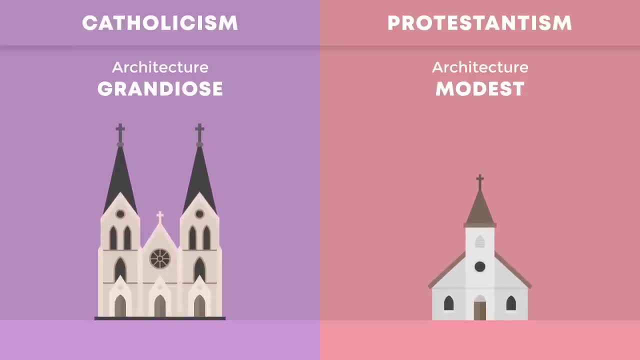 stories, Saints, angels and scenes from the life of Jesus. Protestant churches, in contrast, generally adopt a simpler, more modest architectural style. there's an emphasis on the pulpit and the spoken word, reflecting the Protestant focus on scripture and sermons rather than on visual representations of the divine. 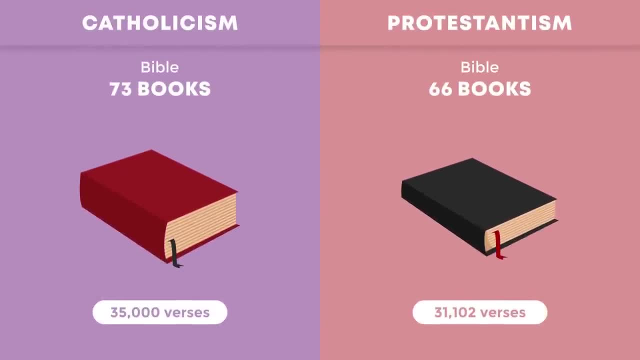 the Catholic Bible contains 73 books, including the 46 books of the Old Testament and the 27 books of the New Testament. these include several deuterocanonical books not found in the Protestant Bible. in contrast, the Protestant Bible, which was a product of the Reformation, is based on the sixty. 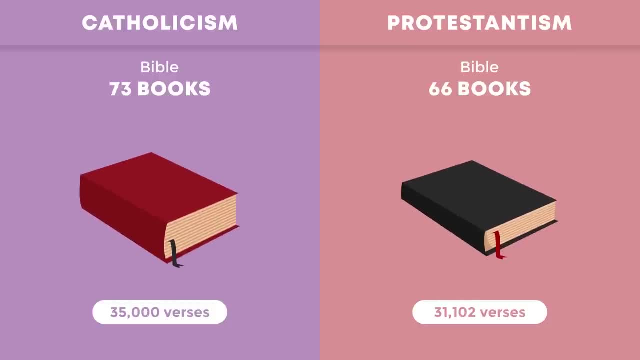 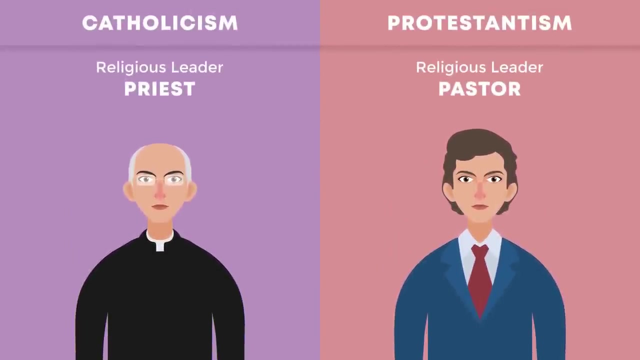 six books that are in the Jewish canon, composed of 39 Old Testament books and 27 New Testament books. it omits the seven books of the Old Testament that Martin Luther and other reformers considered apocryphal. in Catholicism, a priest who leads a modest celibate life is the typical religious leader priests. 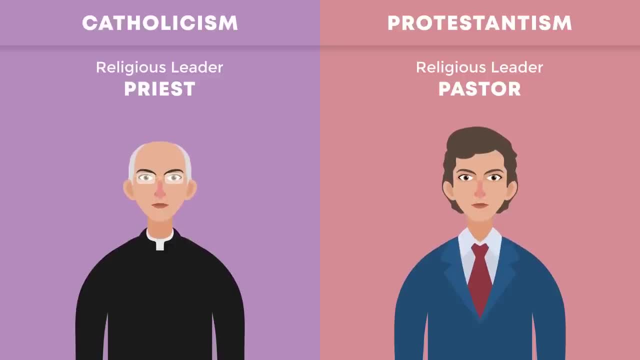 mediate between God and humans, conducting the sacraments and guiding their congregations on the path of spiritual growth. in Protestantism, pastors or ministers are the spiritual leaders. they can be charismatic, influencing their congregations through their personality and teaching. unlike Catholic priests, Protestant clergy are allowed to marry. 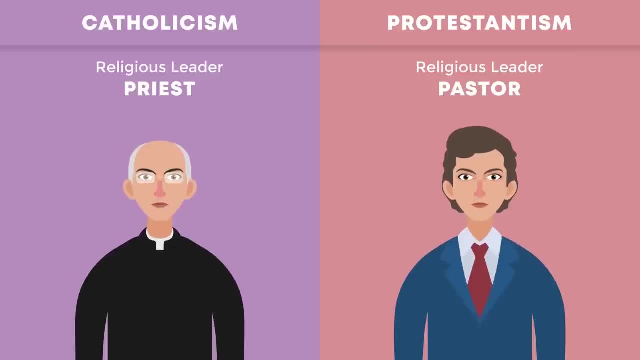 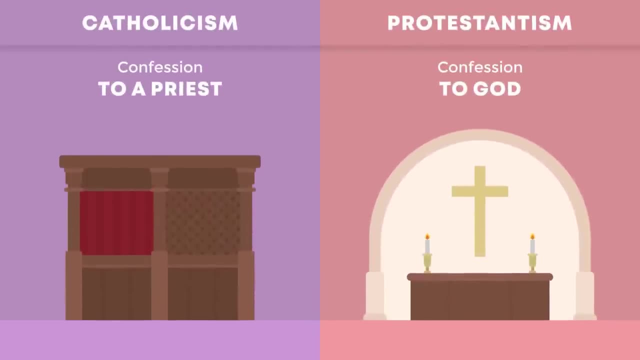 and have children, reflecting the belief that ministers can better guide their congregations if they share the same life experiences. for Catholics, the act of confessing sins is typically performed with the priest within a confession booth or confessional. this sacrament, known as reconciliation or penance, signifies the sinners repentance and God's forgiving grace transmitted. 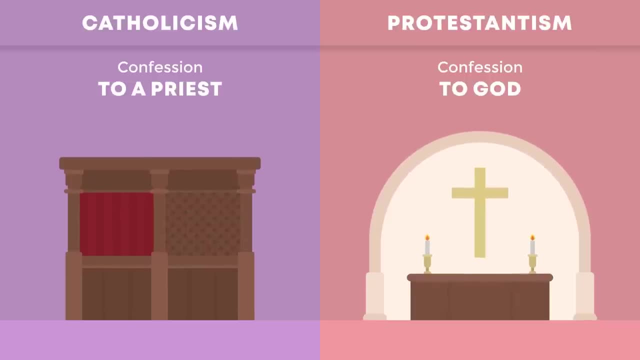 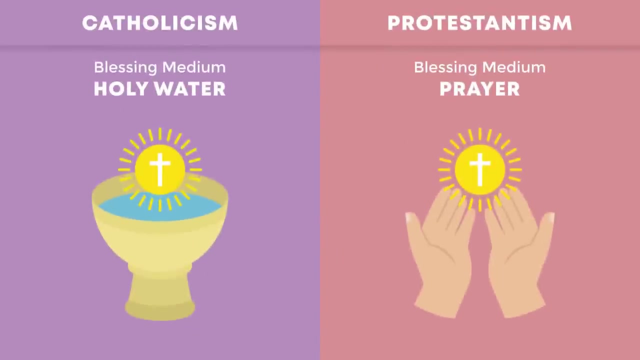 through the priest. Protestants, however, believe in the priesthood of all believers, meaning every believer has direct access to God. therefore, they confess directly to God, believing that forgiveness comes straight from God and doesn't require a priestly intermediary. Catholics often use Holy water blessed by a priest as a medium for blessing. it's sprinkled on believers. 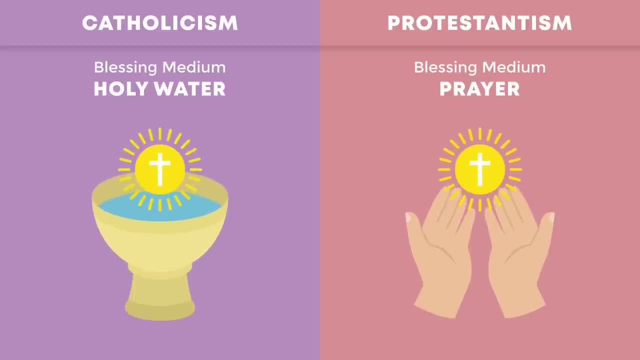 and objects as a sign of sanctifying grace and is used in various sacraments and liturgies. Protestants typically don't use physical mediums for blessings. they believe in the power of prayer alone to seek God's blessings, demonstrating the direct relationship between God and the believer. the use of 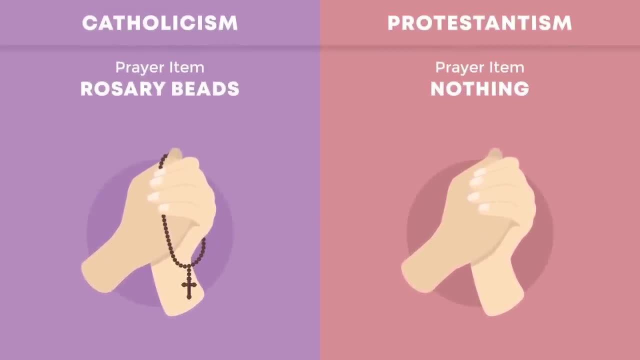 physical items in prayer varies between the two denominations. Catholics traditionally use rosary beads, a circular string of beads for counting the series of prayers that make up the rosary. each bead represents a specific prayer and the cycle of prayers is thought to bring the worshiper closer to 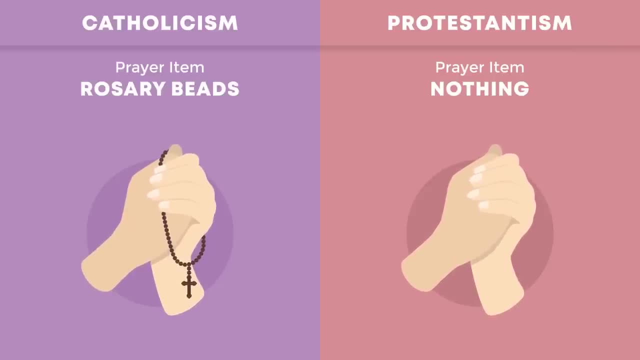 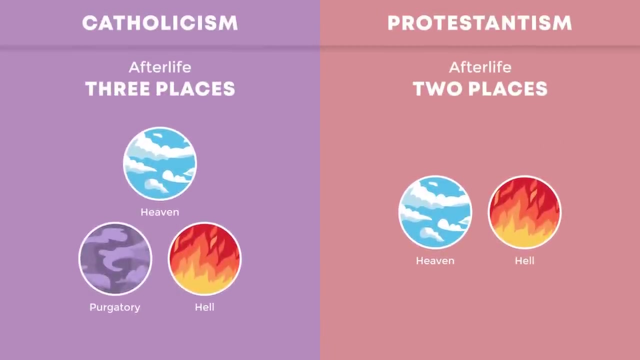 Mary and Jesus. Protestants typically do not use physical items during prayer. this practice underscores their belief in a direct personal relationship with God, unmediated by physical objects or human intercessors. Catholicism posits three realms in the afterlife: heaven for those who die in a. 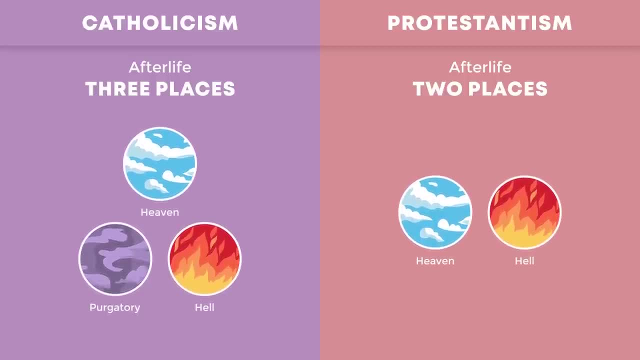 state of grace, hell for those who die in a state of mortal sin, and purgatory a transitional state for those who need purification before entering heaven. Protestant belief, by contrast, usually only acknowledges heaven and hell. the concept of purgatory is generally rejected, as many Protestants believe in. 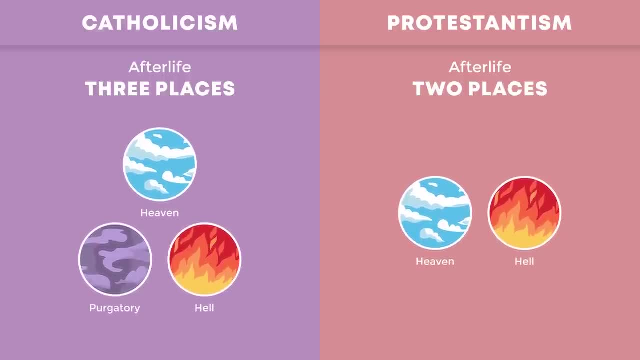 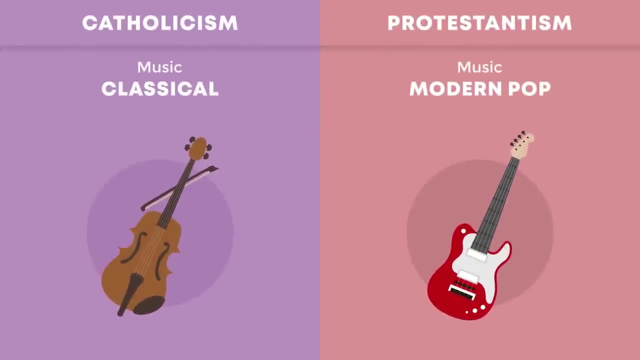 the justification by faith alone, meaning believers are saved by faith in the Holy, in Jesus, not by their deeds. Music in Catholic worship is often slow and calming, frequently using traditional hymns and chants that have been part of the church's liturgy for centuries. 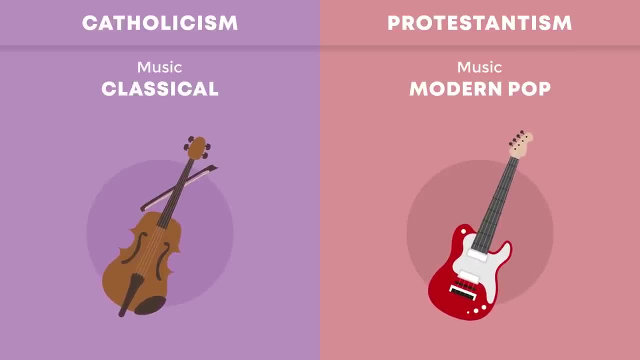 This reflects the solemnity and deep historical roots of Catholic worship. Many Protestant denominations, particularly evangelical and Pentecostal ones, use modern music styles like pop and rock in worship. This uplifting music is intended to inspire congregations and make worship a joyful emotionally. 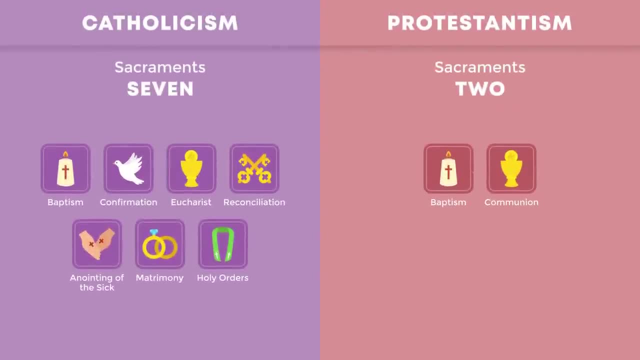 engaging experience. The Catholic Church recognizes seven sacraments—baptism, confirmation, Eucharist, reconciliation, anointing of the sick, matrimony and holy orders. These are seen as channels of divine grace through which believers receive spiritual. 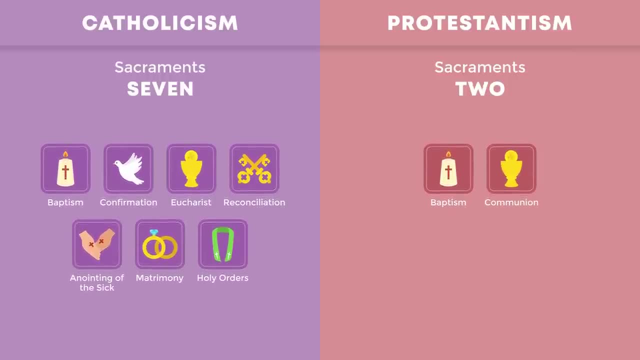 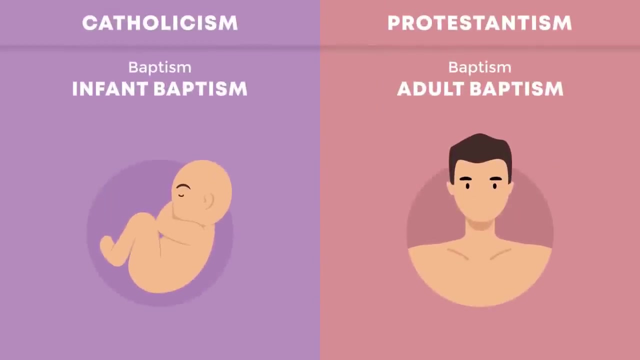 life and growth. Protestant churches, however, usually recognize the sacraments of the Holy Spirit as the only two sacraments—baptism and communion. These are considered ordinances or symbolic rituals commanded by Christ rather than means of grace. Catholicism practices infant baptism, a tradition dating back to the earliest centuries of the 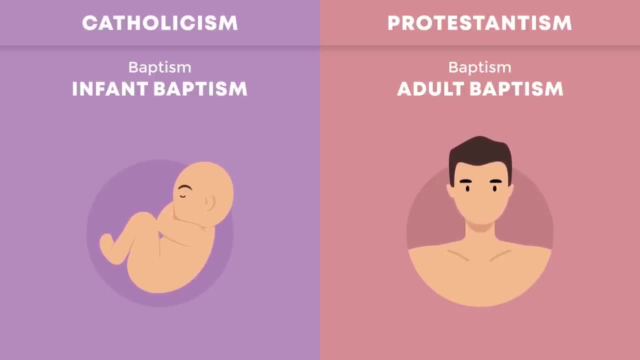 Church. It's based on the belief in original sin and the idea that baptism cleanses the soul and opens the way to salvation. Most Protestant denominations, on the other hand, practice infant baptism as a form of baptism. They practice believer's baptism, or credo baptism, which is performed only after a person. 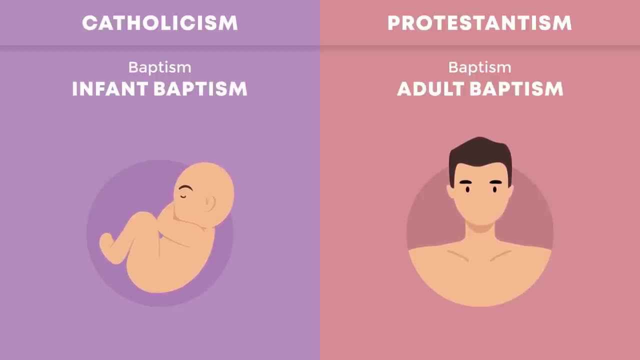 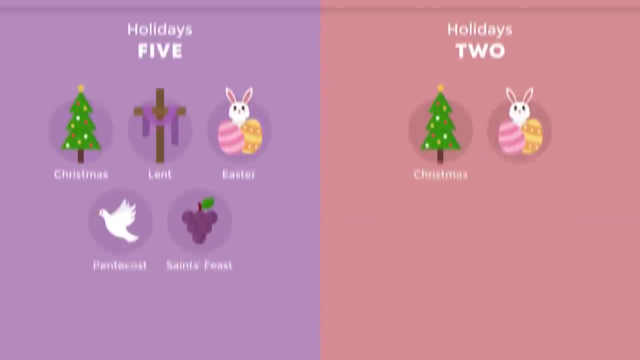 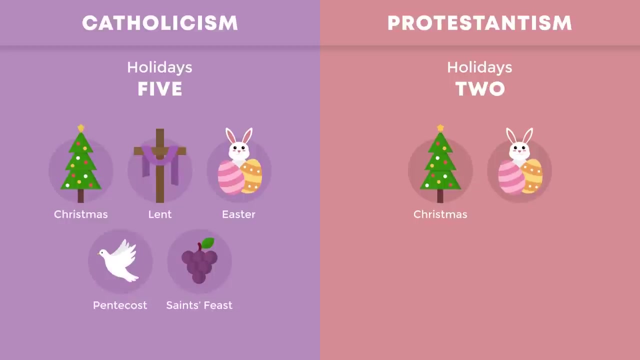 has made a personal decision to follow Christ. They view baptism not as a means of salvation but as a public declaration of faith and identification with Christ. The Catholic liturgical year includes many holy days and seasons. Five of the most significant are Christmas, the birth of Jesus, Lent, a season of penance. 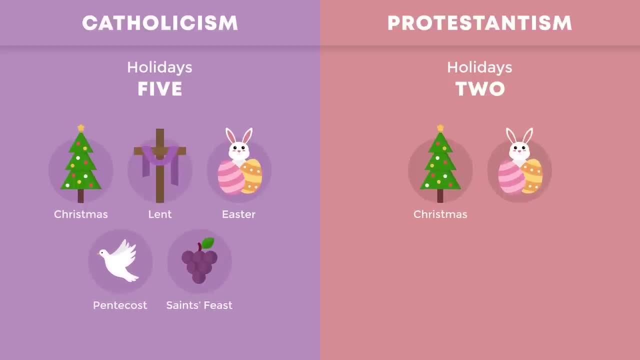 leading up to Easter Easter, Easter Easter, Pentecost, The coming of the Holy Spirit and the Feast of Saints, celebrating saints recognized by the Church. Protestants typically focus on two major holy days—Christmas and Easter—celebrating the birth, death and resurrection of Jesus Christ. 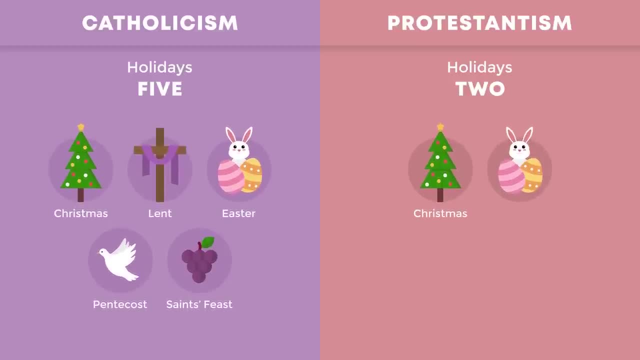 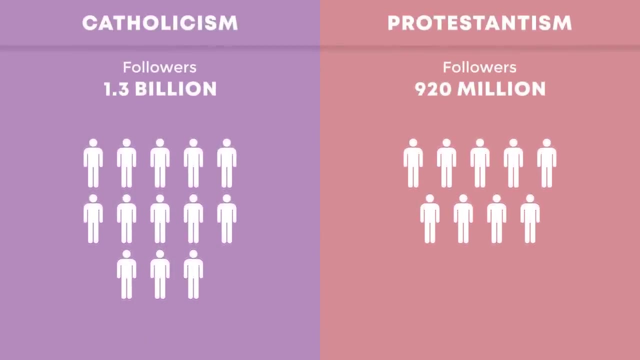 The differences reflect variations in tradition and the relative emphasis on the Church calendar. Catholicism has approximately 1.3 billion followers globally. The Catholic Church has a total population of more than 2,000,000.. This is not a superstition. 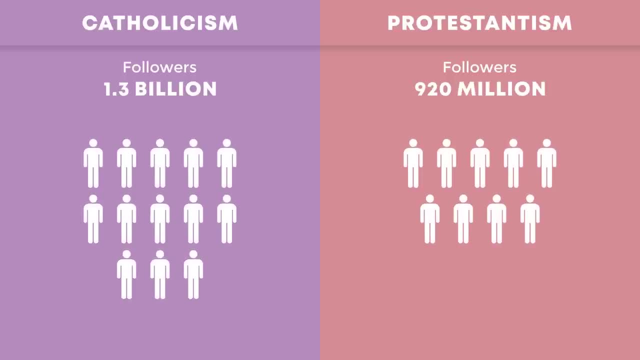 globally, making it the largest Christian denomination. These followers are spread across all continents, with substantial populations in Europe, the Americas and Africa. Protestantism, in contrast, boasts between 920 million to 1 billion adherents worldwide. The movement is particularly strong in North America, Europe and parts of Africa and Asia. 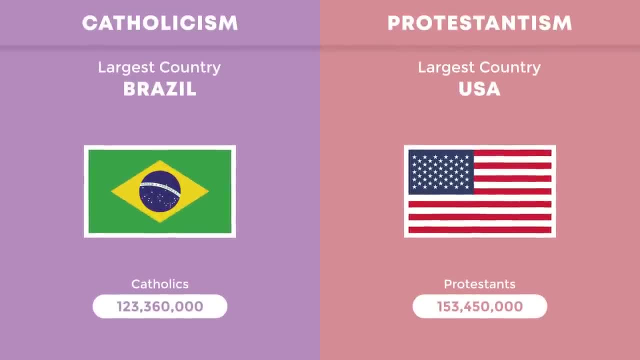 When it comes to the largest country by the number of followers. Catholicism's most significant presence is in Brazil, with around 123 million Catholics. due to the country's historical ties with Portugal and its missionary activities, The United States is home to the most substantial number of Protestants, approximately 153 million.